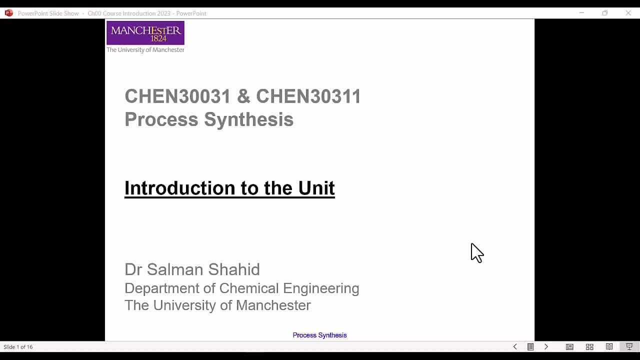 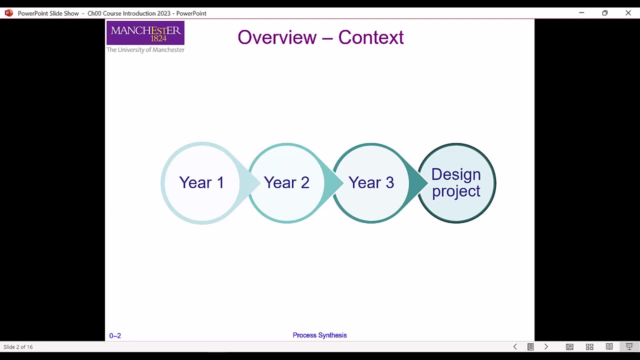 To understand this, we will use what you have learned in your degree so far and what you will be learning in this semester. So the design project which you will carry out in the next semester is sometimes known as a design project. It is a process that you will be using as a capstone course or a project in your degree, in which you normally use a full set of knowledge that you gained so far in your program. 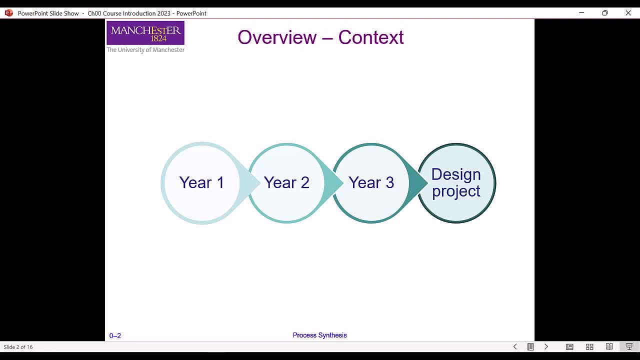 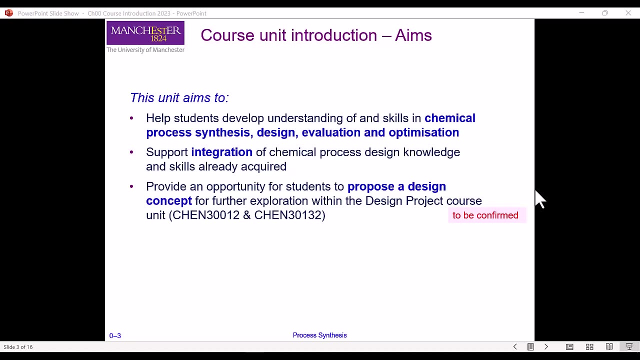 And process synthesis is highly relevant to your design project and to your integration of knowledge and skills from the degree program so far. So the aims for this project are to help you develop an understanding of what a chemical process synthesis is, How we can design that process and then look into the evaluation and optimization of that finalized design. 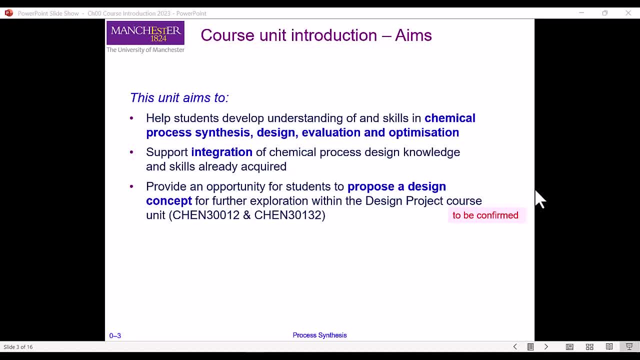 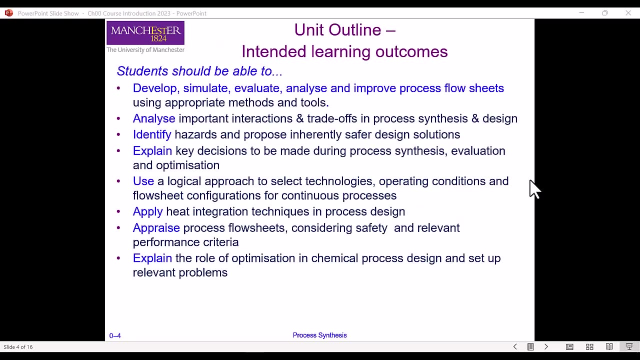 This unit will also serve as an opportunity for you to propose a pitch project that you can. you want to do it in the next semester? Okay, but there will be more detail provided about it in the coming lectures. So this slide provides you the unit's internal learning outcomes. 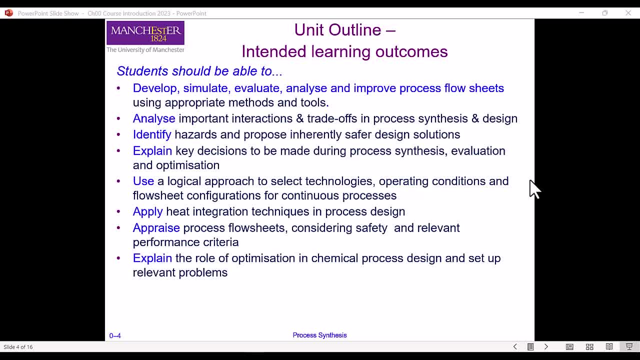 And you can go through them in your free time. And once you go through them, hopefully you will realize that this unit is not all about doing calculations, but also about analyzing flow sheets, explaining design decisions, applying logic and considering multiple performance issues. 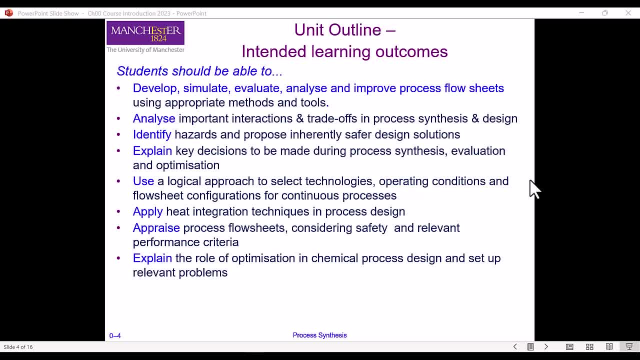 And these kind of learning outcomes require you to be able to make sense out of your calculations, And they also require you to be able to consider qualitative issues, trade-offs and sometimes in situations where there is very little information is available. And we will practice these concepts and ideas in lectures, tutorial sessions and problem sheets. 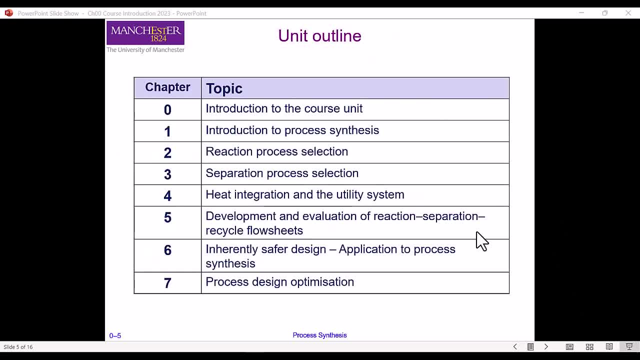 This unit consists of mainly seven topics, And chapter zero is We will discuss mostly the revision of the concepts that you have already learned. Then we will go through the introduction of the process synthesis. We look at reaction separation and heat integration, And then we look at alternative forms of flow sheets. 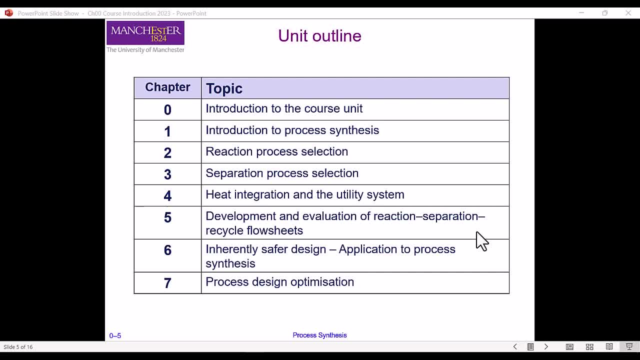 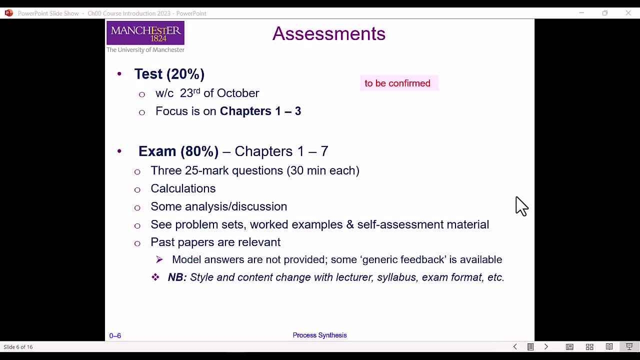 And finally, in the last two chapters, we look at safer design and how we can optimize our process. So, in terms of the assessment of this unit, so we will have two types of assessment. We will have an online test that will account for 20% of your final grade. 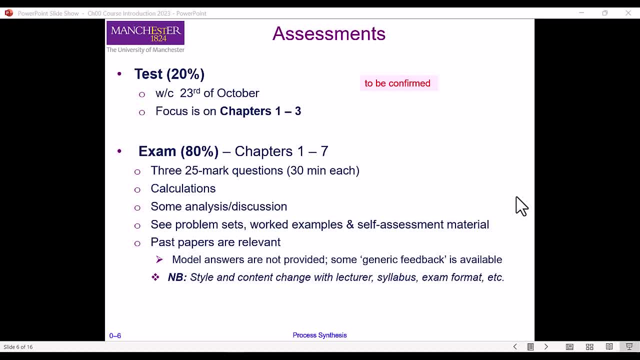 It will cover chapter one and chapter two, chapter three, And it will be in week commencing 23rd of October- Okay, but this is still to be confirmed And we will have a final exam that will account for 80% of your final grade. 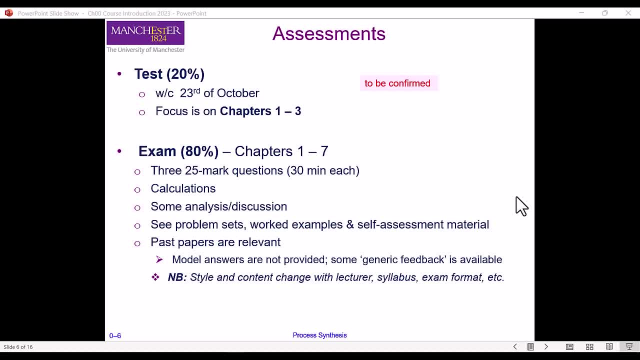 And unit grade and it will cover chapters one to seven. You will have three questions, each for 25 marks, and you will have in total two hours to solve that exam. And the questions in exam would be around calculations Like, for example, designing a system or analyzing a process and discussing a particular scenario. 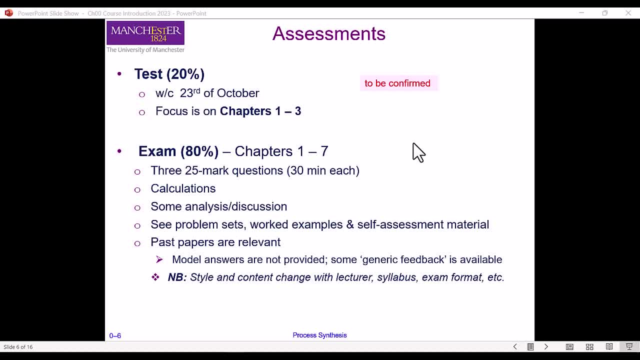 And we will practice these questions or these concepts in our tutorial sessions and also in our problem sheet And also on Blackboard. if you have a look, there is a folder called exam preparation that contains the exams from past few years And the answers are not provided so you can try to solve them as you move along this unit. 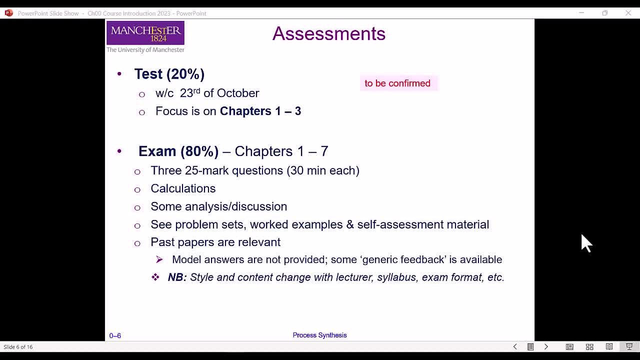 Please be aware that the flavors has changed with time And in personal as well, So if you see some questions that seems very far from what you have been learning this year, then it is quite likely that the unfamiliar material is no longer in the syllabus. 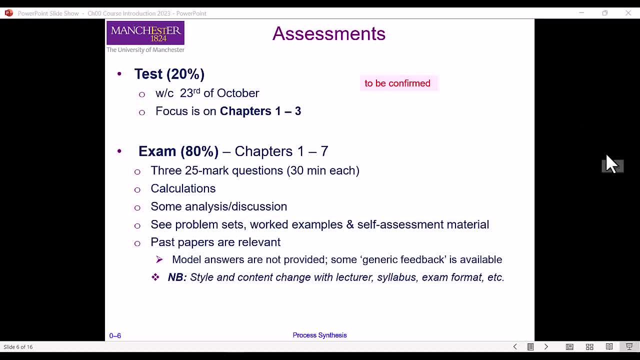 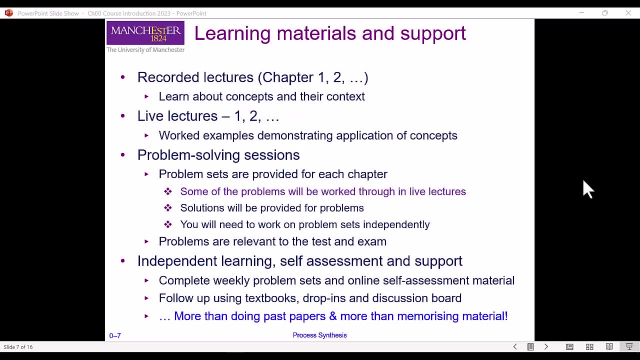 Okay, so please remember that. So this unit will be delivered in blended learning. It means that some part of the material would be delivered online and some part will be in person. The core concepts will be delivered in pre-recorded asynchronous video format that you should watch before you come to the corresponding synchronous session. 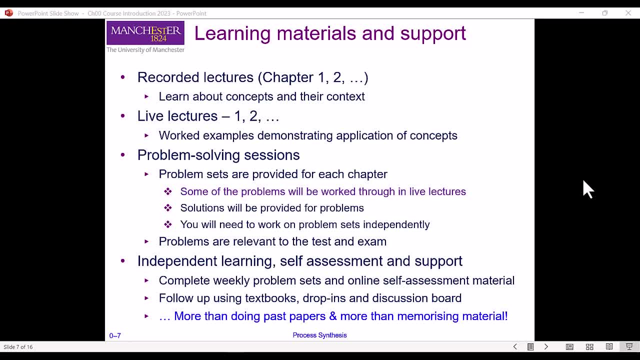 Okay, where we will go through some work problems and exercise problem sheets. My aim is to have the chapter material available to you by the week before timetable session on Monday. Okay, so some material in this unit can seem quite abstract And I think that the application of the concept is really helpful for developing an understanding of more abstract concepts. 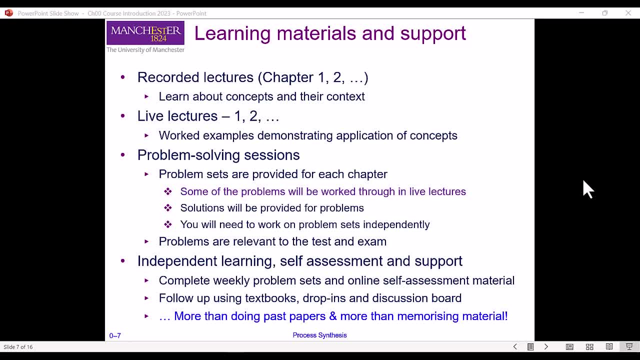 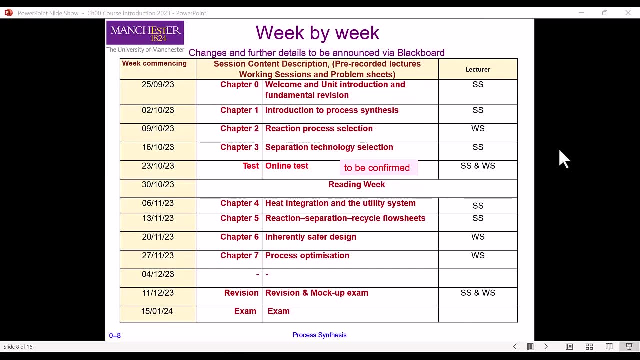 Okay and that we will be doing in the tutorial sessions. The problem sets for each chapter are very important and they are actually the main way for preparing for your test and the final exam. So this is the plan for next 10 or 11 weeks. 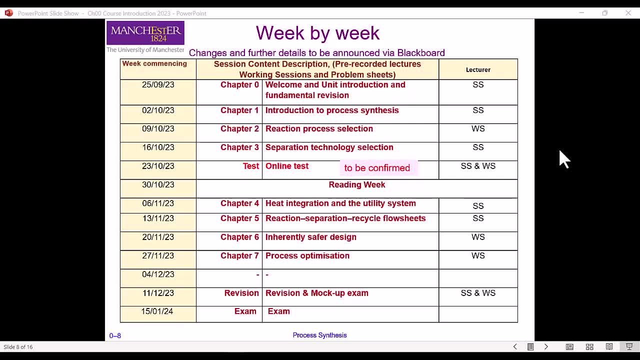 Most weeks we will work through one chapter of the taught material And most of this taught content is covered in pre-recorded lectures. The live lectures will present working sessions where we will go through some problem exercises, as I said in the previous slide, And we will look at how we can apply concepts. 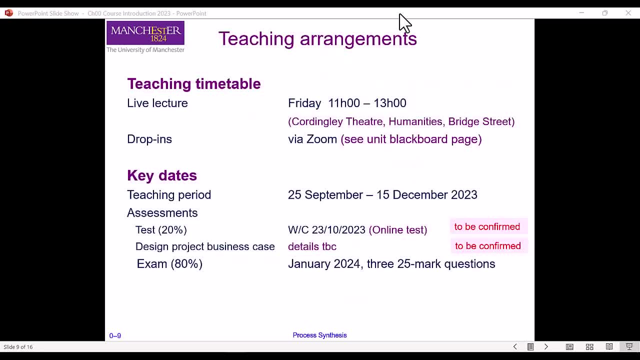 And approaches covered in the chapter. The sessions for this unit should be booked in your timetable. Okay, so it's every Friday from 11 to 1, and in accordingly, Theatre Humanities, Bridge Street, And for the drop-in sessions. we will do it remotely using Zoom. 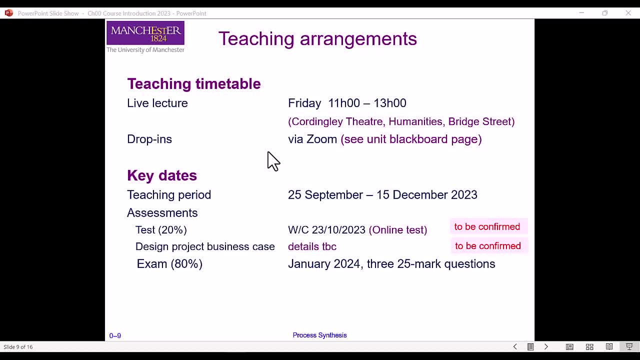 And the link for the Zoom meeting would be provided on Blackboard page. Okay, Here you can also see some key dates for this semester and for this unit. The most important here is that the exam, the online tests, would be in the week of 23rd of October. 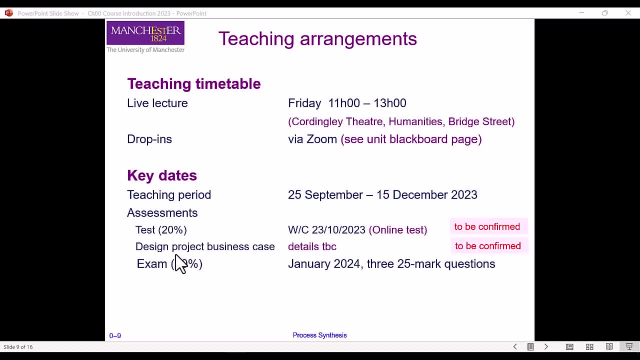 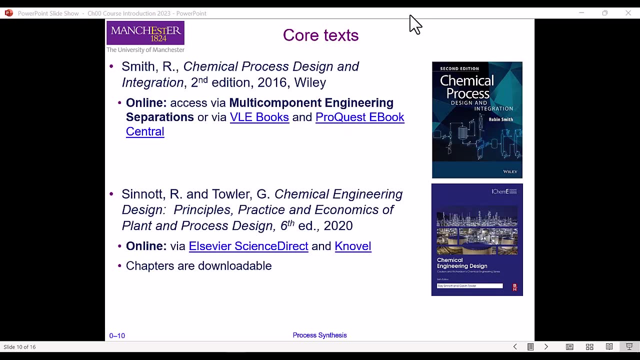 Okay, but this is still to be confirmed, And also that the design project business case pitch date- that is still to be confirmed. Okay, We will be using a couple of textbooks for this unit. The textbook by Robin Smith is a core text for this unit. 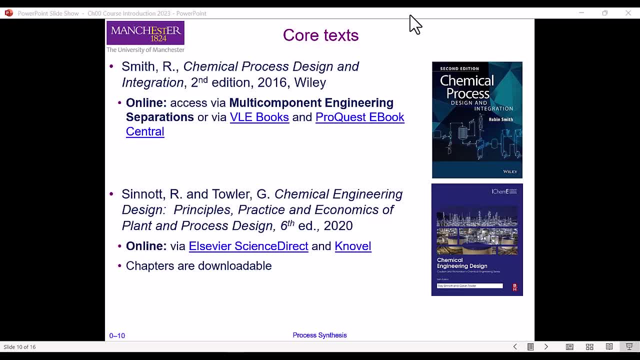 If you have access to it via multi-component engineering separations, you can download it completely and save it indefinitely. Okay, And I would recommend you to do that. If you access the same book via library, you will be directed to VLE books or ProQuest. 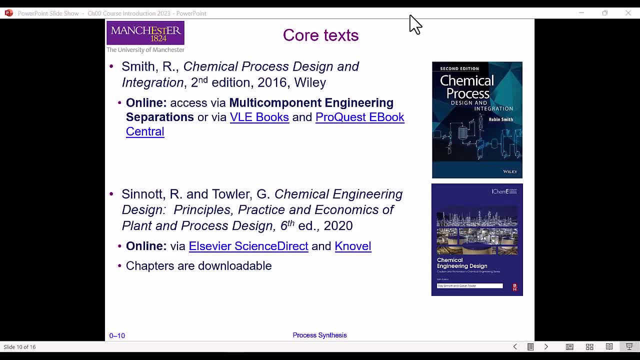 And then you can only read or download a part of this book, Okay, And that part also will expire after a few days, So preferably try the first option, Okay, And the other book is Chemical Engineering Design by Sinnerton Towler. 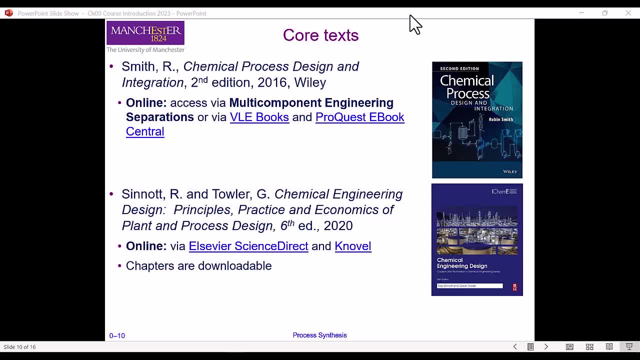 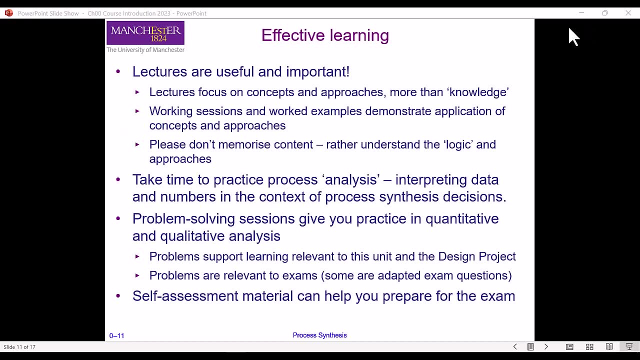 And that is another very valuable journal design related resource that you can use. You can access this book via library And that is not restricted. Okay, So you can keep it in your system. This slide emphasizes that there aren't easy shortcuts to succeeding in this course unit, because of the higher level of learning outcomes that are needed. 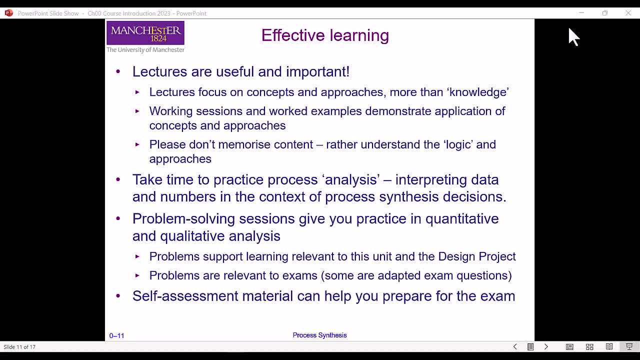 So please don't waste your time in memorizing the content. It's far more important that you develop understanding of underlying concepts and then applying logic to solve unseen problems. Okay, The problem sets should be valuable in developing the relevant problem-solving skills. 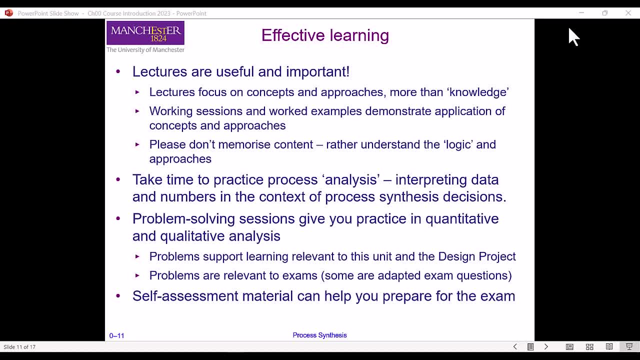 And also they will help you to prepare you for exam problems. Okay, And also, please remember that this unit follows on from and integrates knowledge from earlier units and develops concepts that are vital for your semester 2 design project. Okay, So please don't consider this unit as a stand-alone unit. 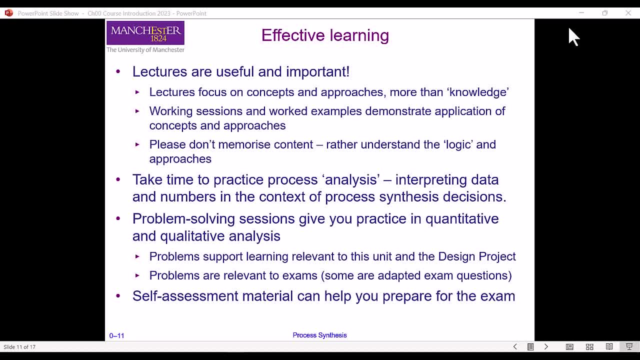 You will be using the concepts that you have learned already, But now you will be more in a position of making changes. So you will be the designer that has control to change things. You will be able to change the process conditions, compared to year 1 and year 2, when you were given the problem and you had to just solve it, but you were not allowed to change the conditions. 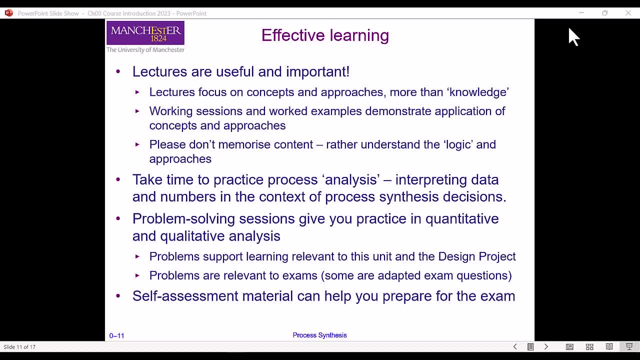 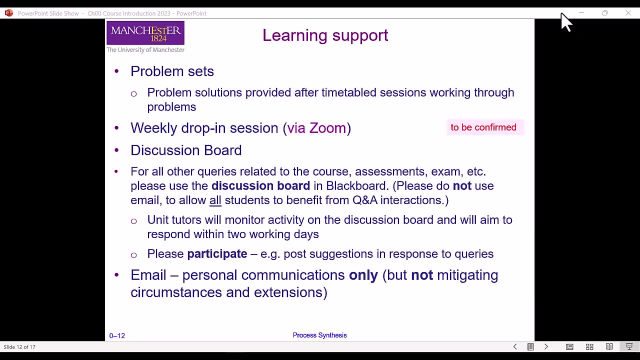 This unit, you will be a designer that has the flexibility of changing the parameters of the process to make the best use of the process. So, to help you with the learning, the problem sets are designed to allow you to apply concepts developed in the lecture materials. 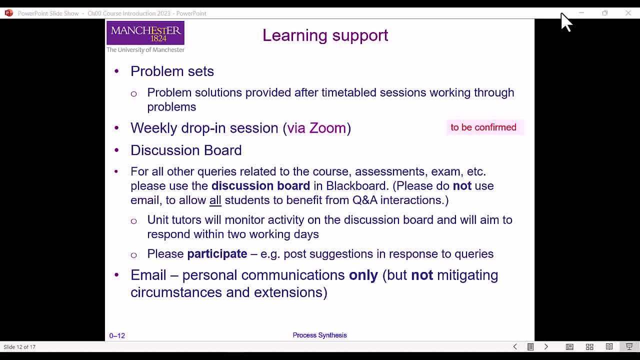 So working through these problem sets is therefore crucial for you to prepare for the exam. Okay, In addition to live lectures or problem sets, you will also have drop-in sessions where you will have the opportunity to raise questions about material problems or any concepts that are not clear. 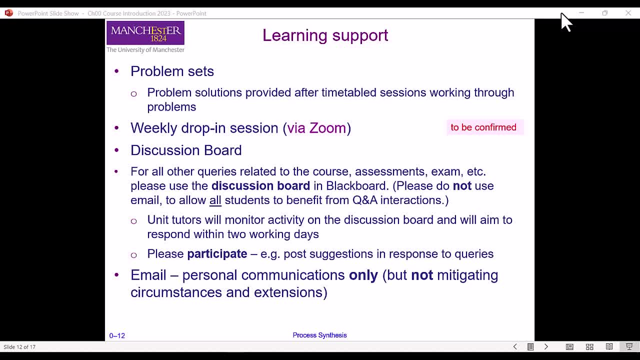 Okay, We would like to use discussion board as far as possible to respond to your queries in this course. Please use discussion board because it will allow others to learn from your questions as well. okay, or the answers you get. Also, you are encouraged to answer queries posted by your classmates. 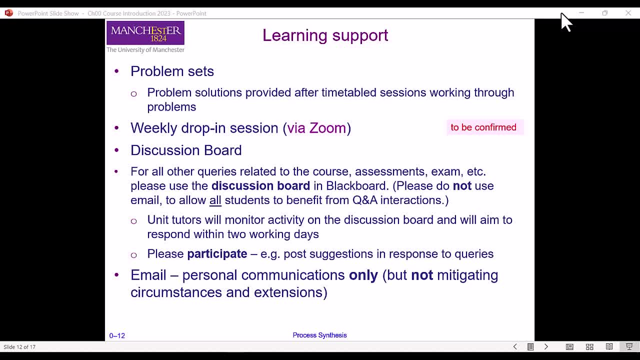 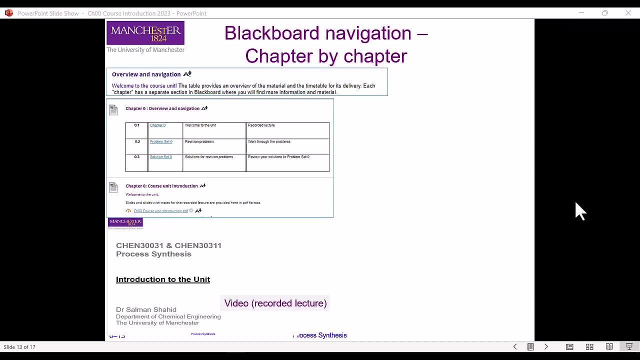 We will keep an eye on the responses and give you a gentle steer if the response is incomplete or misleading, But otherwise we would very much encourage you to help each other develop the skills and the understanding of a concept. So this slide gives you an idea how the material will be organized on Blackboard for all the chapters. 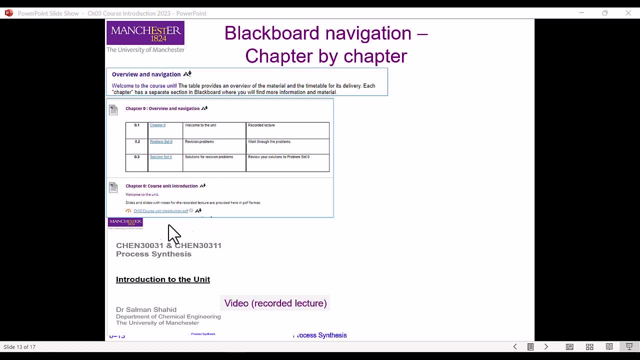 So for each chapter you will have a pre-recorded video available to you on Blackboard and it will be uploaded on Monday, a week before the actual synchronous session, And then, once you have the synchronous session, the forecast from the synchronous session will be available to you on Blackboard in the folder, in the chapter folder. 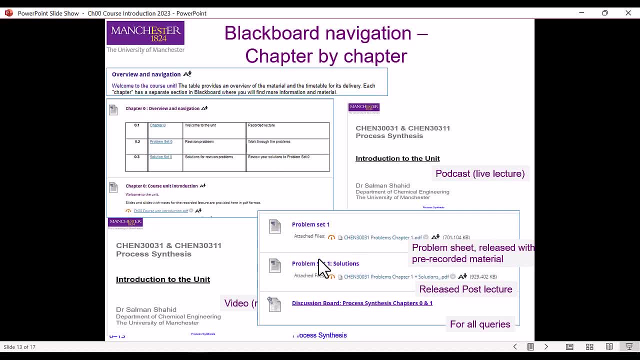 Okay, And finally, you will have the problem sets. So problem set questions will be available to you with the pre-recorded material, but the solutions of this problem set will become available after the podcast. okay, after the live session. So I listed Internet learning outcomes on slide four. 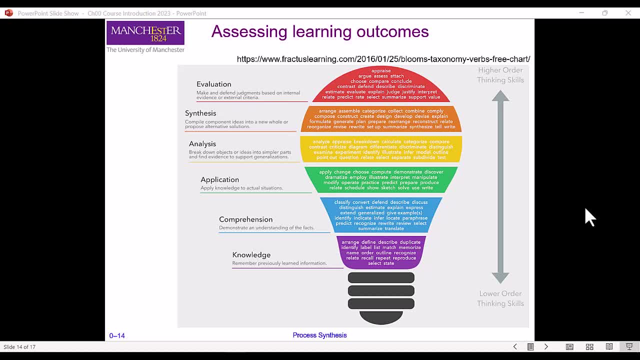 And this slide highlights that learning happens at various levels And emphasizes that the assessment in this unit aims to test your learning at basic as well as higher levels of learning. Okay, After all, this is higher education. At basic, end of spectrum is knowledge such as definitions and understanding of concepts.